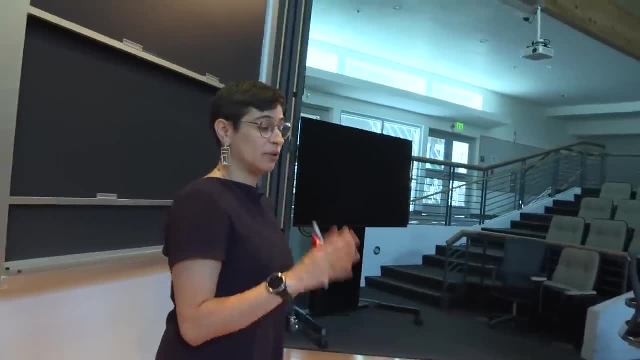 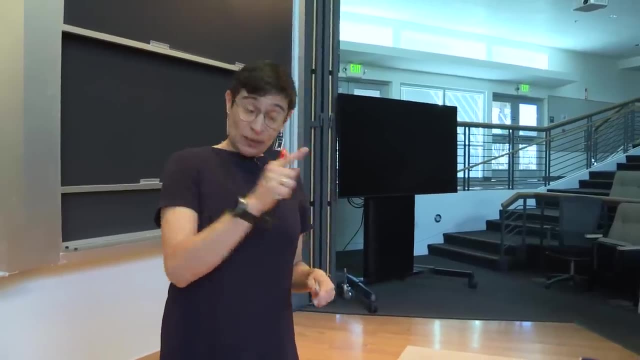 Right, right, right, And in fact you know like. so this is a little bit of a lie, because if you open Euclid's element, you're not going to find this statement the way it is written. So in fact, the way he wrote it is more similar to what you were saying. What he said is: 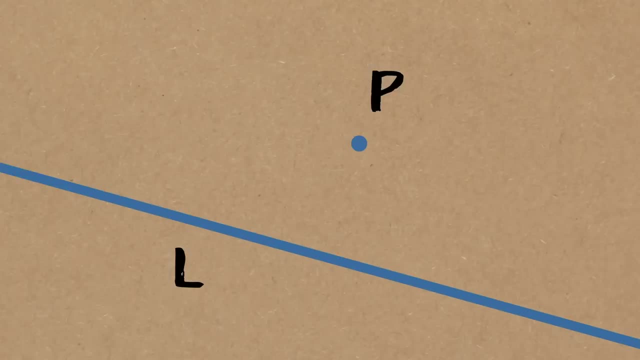 you know, if you have a line and then you have the point P, you draw your line through P. Then let me draw just any other line through P to help. What he said is: the sum of these two angles is less than 180 degrees. Then the lines, once you extend them. 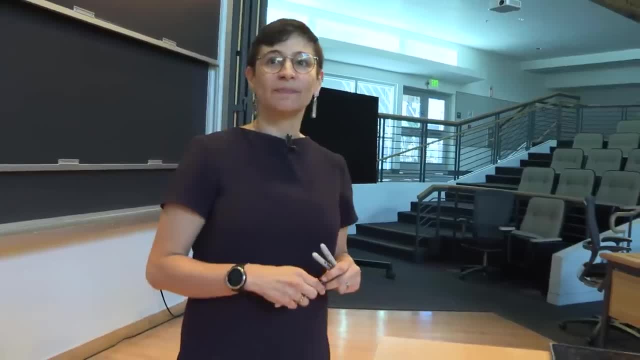 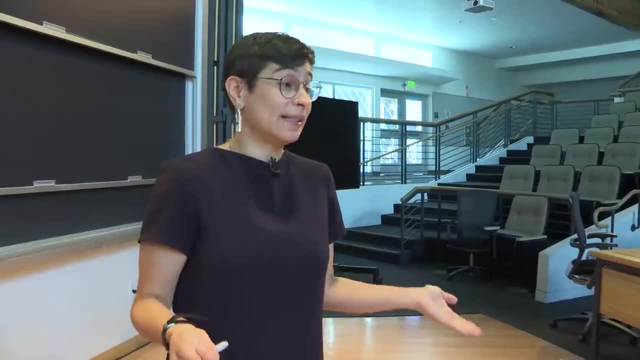 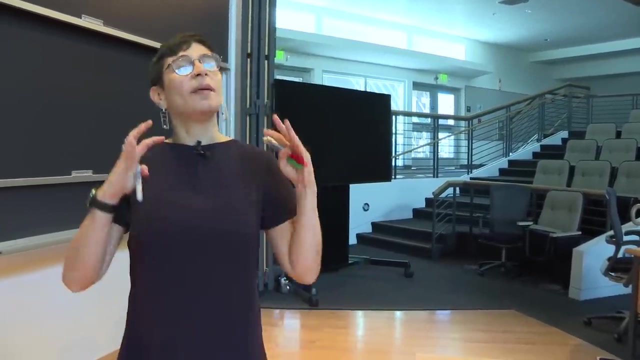 to infinity, they're going to intersect. That classic Euclid parallel postulate seems true to me. Yes, exactly, exactly, And it well, in fact, it seems true to you and to most of us because it is actually true. But it sort of depends on the model of geometry that we're considering right. 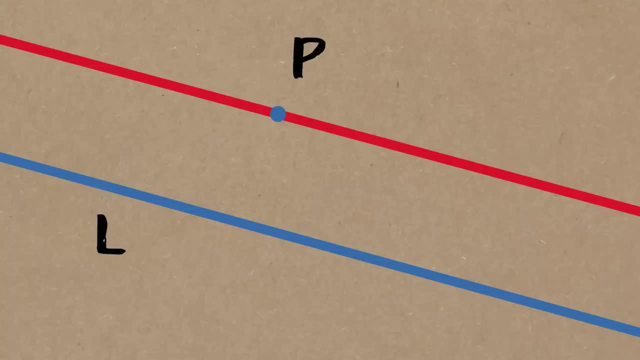 Here we're working on a plane And to do geometry we need, among many other things, a way of measuring distance, And you know like if we're here in the plane, we measure distances with a ruler Or, if you want, you know like there's a formula. 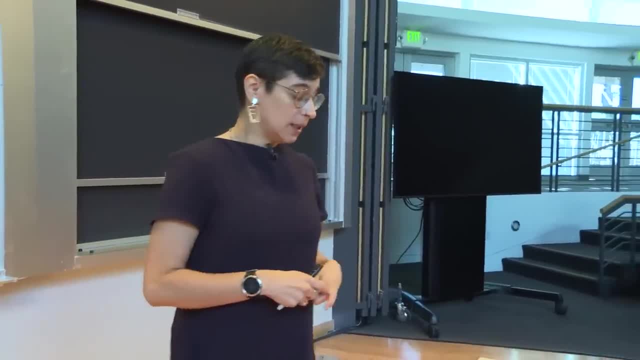 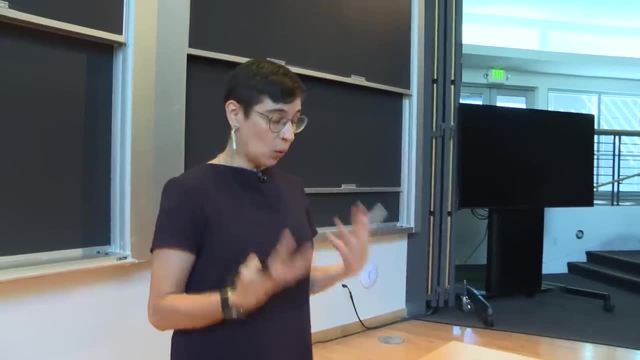 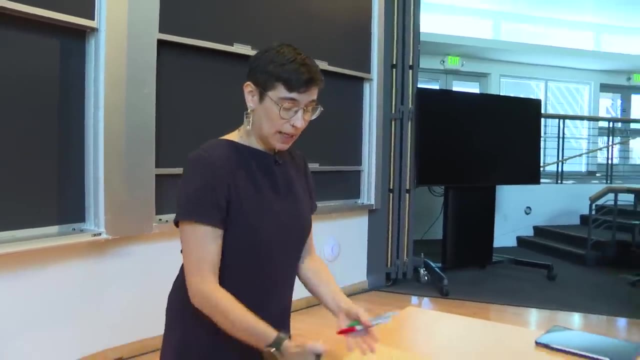 if you have coordinates. it's basically the Pythagorean theorem. So we have, we know what we're doing. However, that is not the only space in which we can do geometry, Not even two-dimensional space, right. So the plane we have a vertical direction. 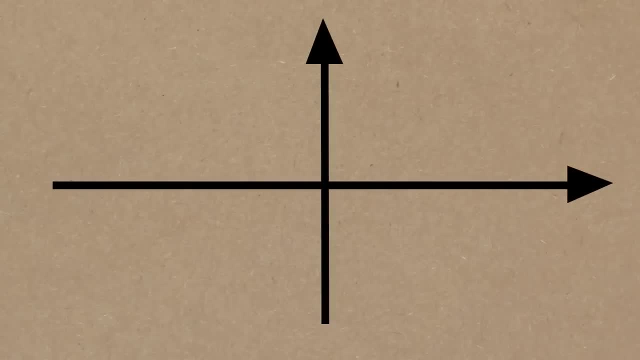 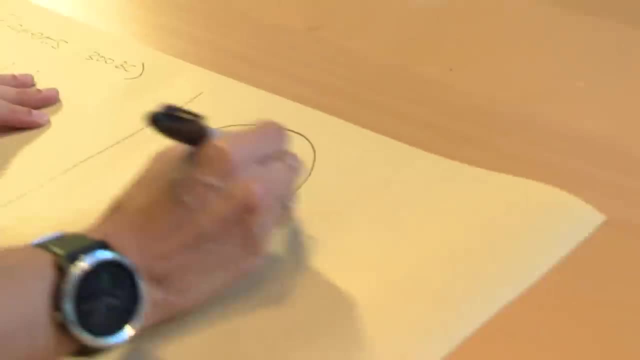 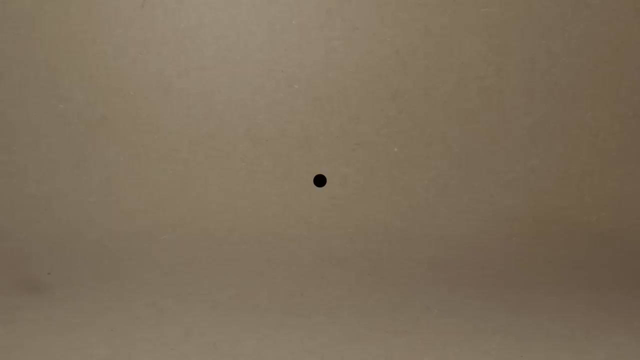 and a horizontal direction. Those are our two dimensions. right, Let me show you another space where we can do geometry. Here's what we call a sphere, So as mathematicians call it as S2, if you're a mathematician, then you draw R3 three-dimensional space. 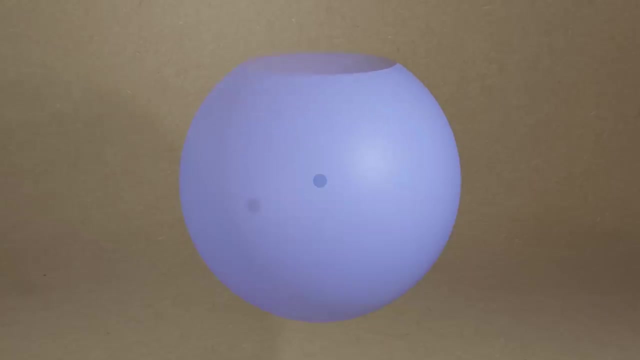 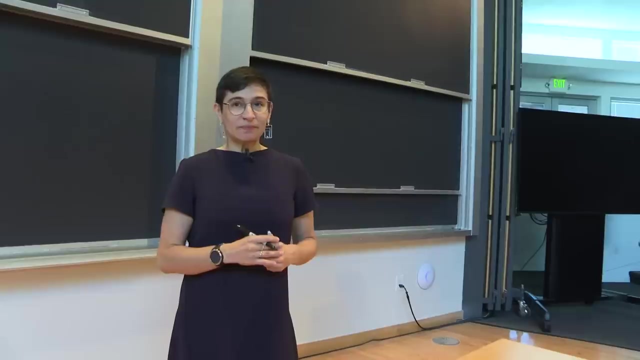 and you say that this is the set of points that are about V right, points that are at distance one from the origin. If you're not a mathematician, you're just looking at the shell of a football ball. Is this a two-dimensional space? This is a two-dimensional. 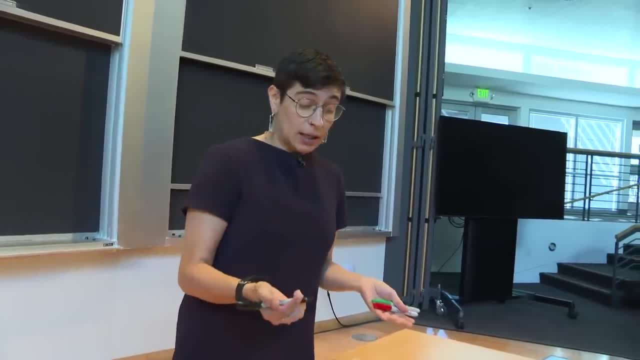 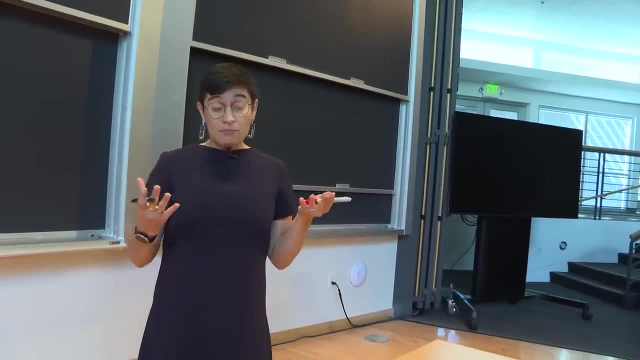 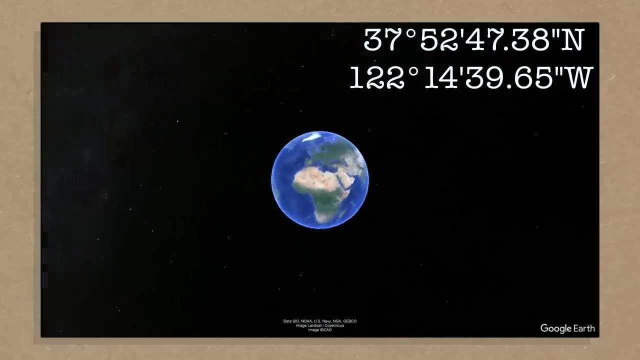 space because, again, we basically only have two directions in which to move right. So, if you want, we can do it in terms of meridians and latitude, right, The way we do it to describe location right, Like if you look in google maps, if you want a precise location, you're going to get two. 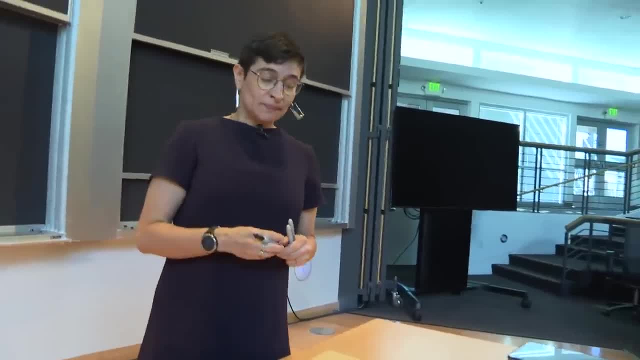 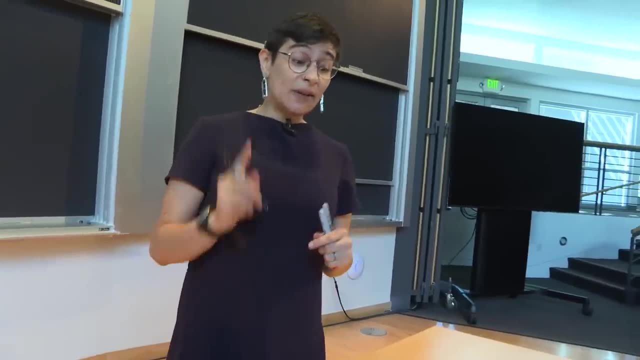 coordinates. Yeah, Exactly that. Okay, so although we think of balls and things as three-dimensional objects, because we're only dealing with the shell, it's a two-dimensional. Exactly, yeah, and that is very important. We're not thinking about the feeling. You know that. we're thinking about 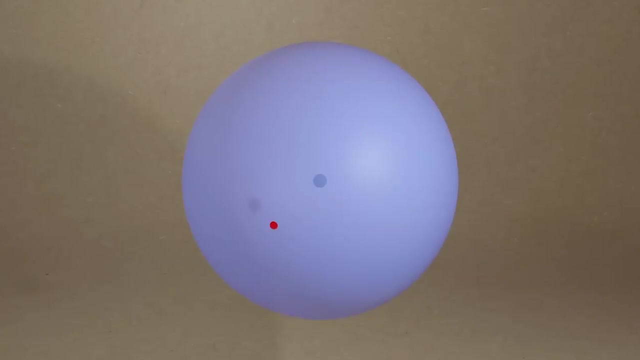 a little ant that is just completely flat. So what happens to the parallel postulate here? Well, so you know, here I started by telling you there's something that's not right. There's something that's not right. there's something that's not right. 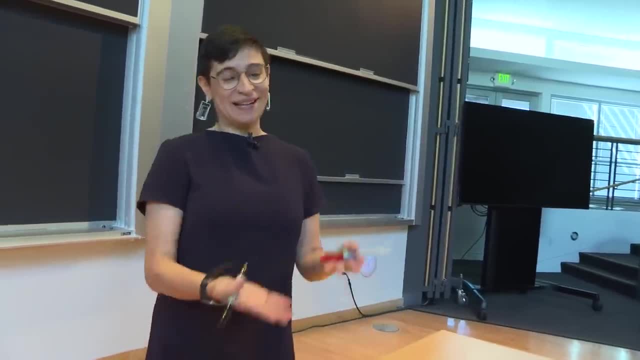 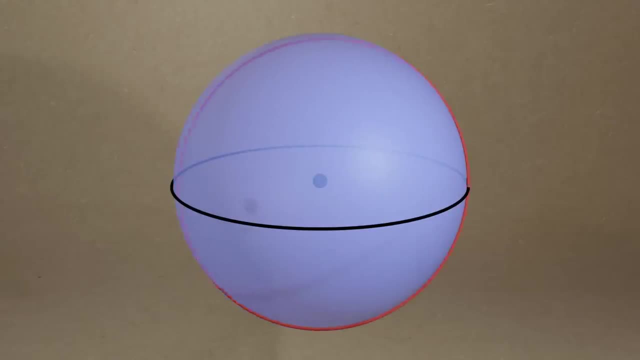 a line and there's a point right. So I have to tell you the same thing here. I have to define my objects. So a line in here is going to be what we call a great circle. What is a great circle? Take the intersection of this sphere with a plane that goes through the origin. So this is a great. 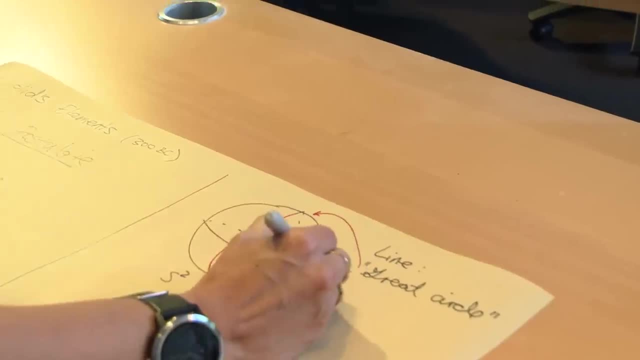 circle, Or you know the way I drew it here. this is the equator. That's also going to be a great circle, So every line has to be the longest possible line, does it? It can't be just a little. 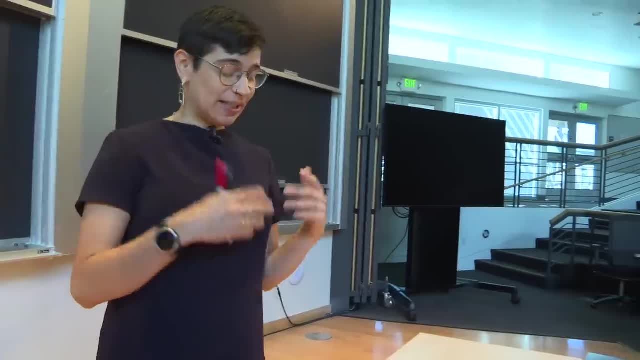 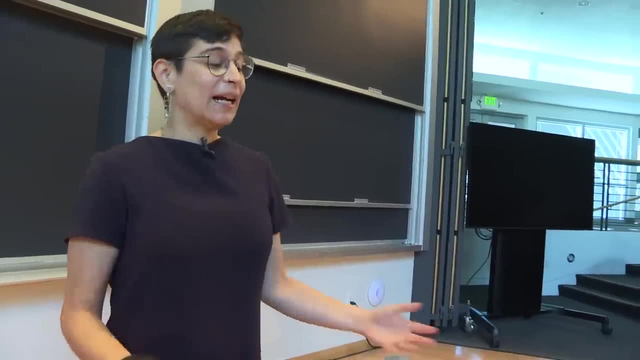 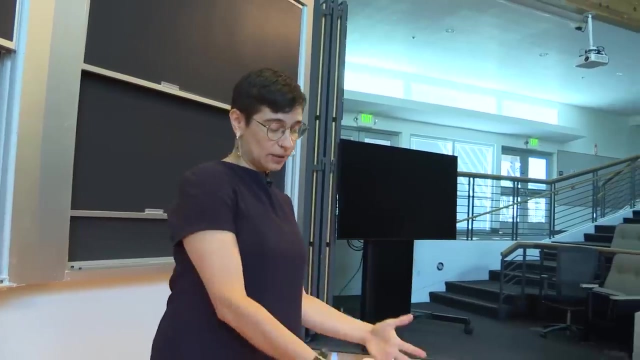 circle. Aha, So this is key, right? So there's a difference between what we call a line and what we call a line segment. right, And actually so that line segments. that's one of the first rules that we have in Euclidean geometry, or in the geometry of the plane, which is that, if I give 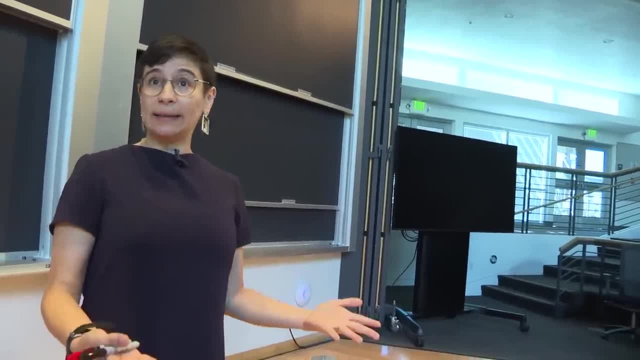 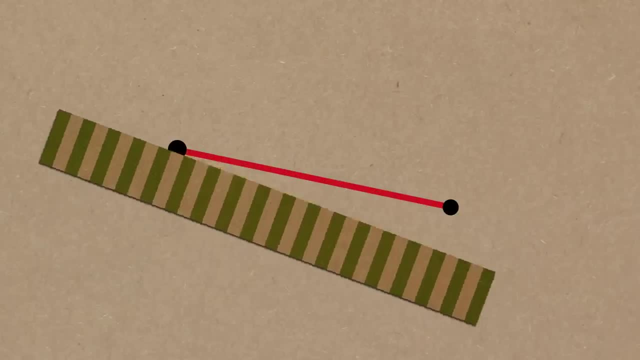 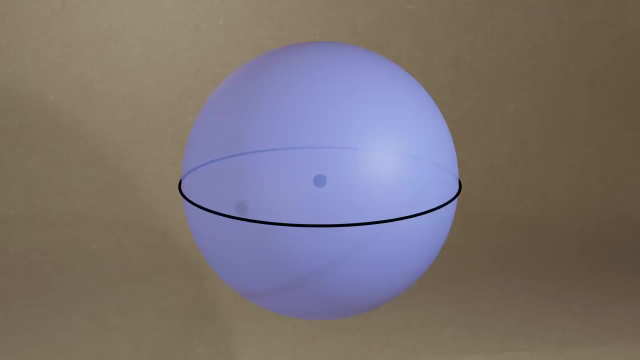 you two points. you're going to be able to give me a line In our plane geometry. that's pretty easy. Two points: we get a ruler. here's the line right. Pretty easy. We know how to do it Here. it's a little trickier but it's not so bad If you choose. 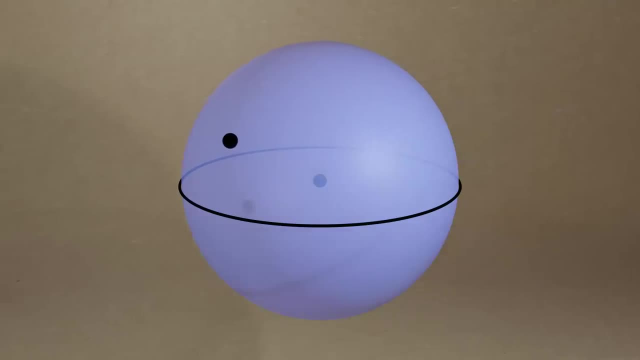 a point, say over here, and then maybe a point over here, then how do I find the great circle that goes through them? right, And I need to find the great circle and then only look at that little segment that connects them And that's. 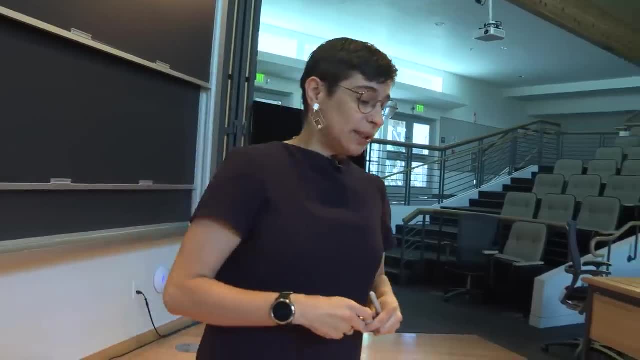 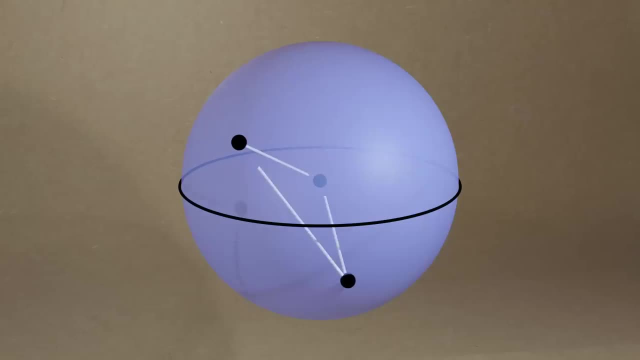 another, that little segment. Well, we can do it by choosing. you know like we can extend these points, join them to the origin. There's a little space in between them. Let me fill that with a plane. That's the plane that's going to intersect my sphere. It's going to be something like that: 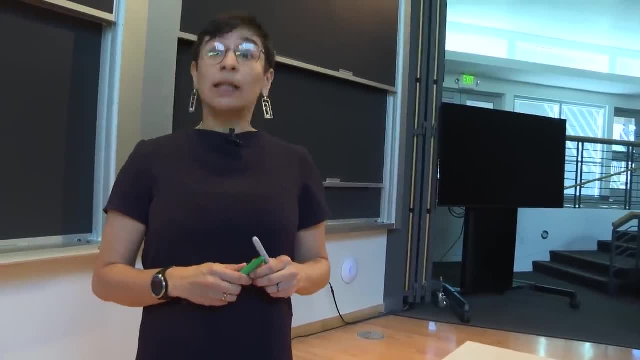 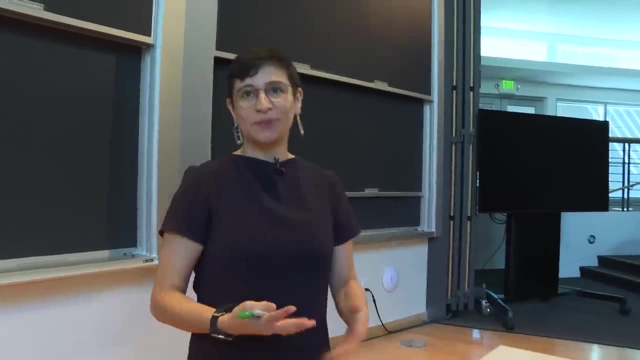 So you're trying to find the equator, basically that on which both of those lines sit, Exactly, Exactly, Except, you know, like it's a tilted equator. right, It's not, But yes, that is basically it. 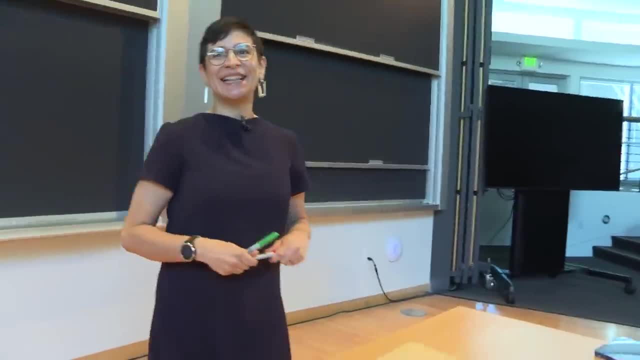 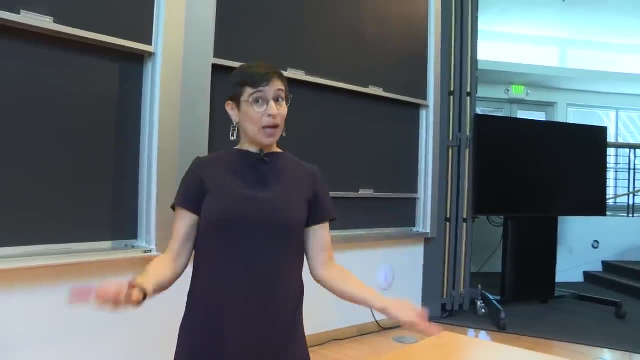 I could have. I mean, I could have cheated and just chosen two points in the equator, But so what I drew here is a line right. So the line segment. Well, we have two options. This very clearly short one, 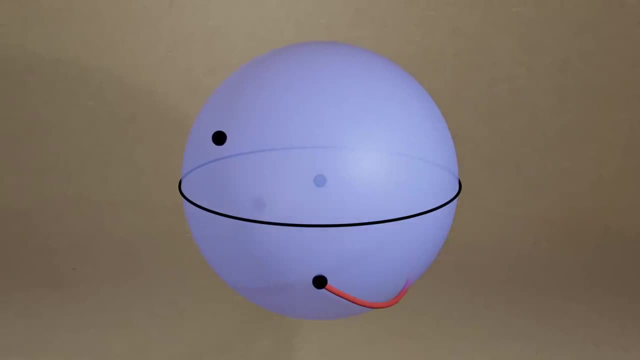 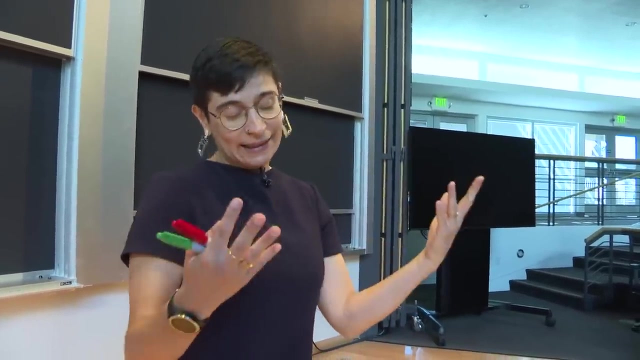 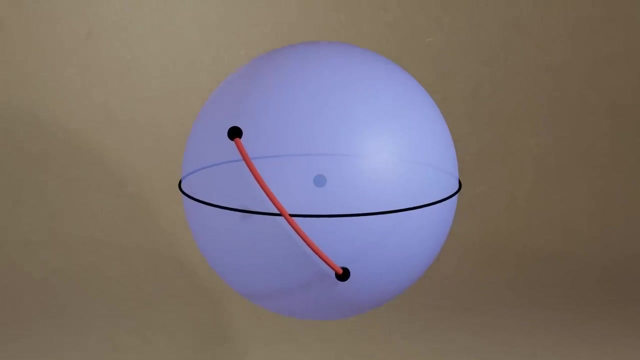 But then there's another one that is longer and it goes around. Sometimes what we say is that a line segment is the segment, that whose length is less than half of the entire circumference. That fixes some issues. So what does this mean for the parallel postulate? 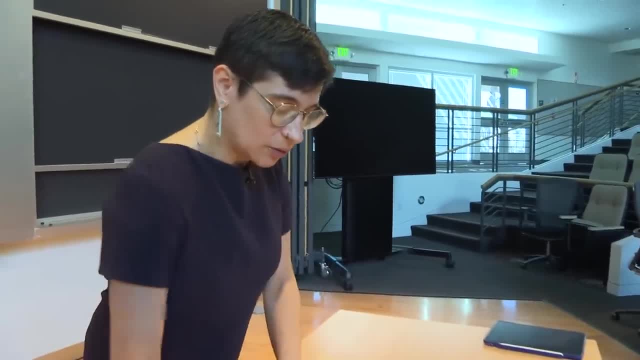 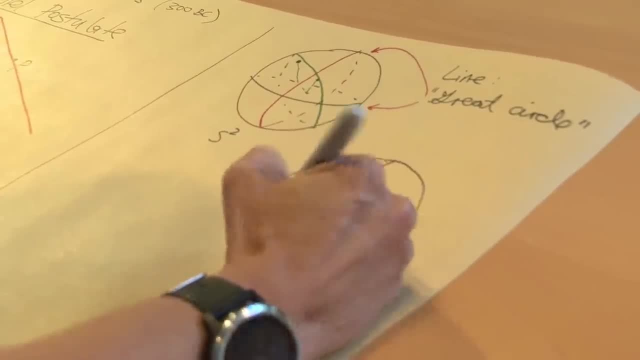 Excellent question. So let me do, let me draw my sphere here again. I'm going to draw a line that is easier for me. Again, this meridian, That's my line. So this is my line L, And then I'm going. 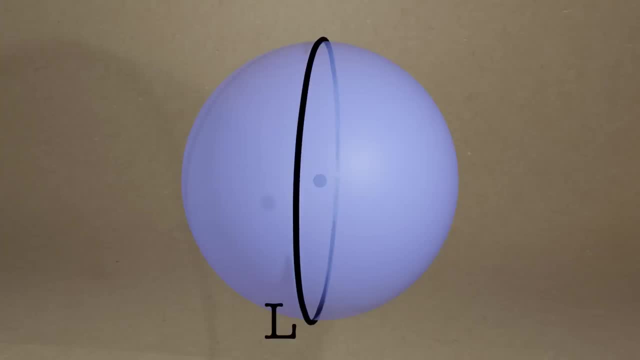 To get my point P, Let me choose this point P right. So lines that go through P: There's this one. Here we have a problem, right, We have this intersection, this intersection, So maybe we need another one right. 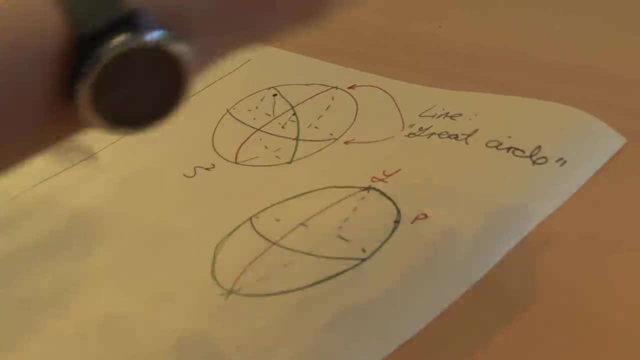 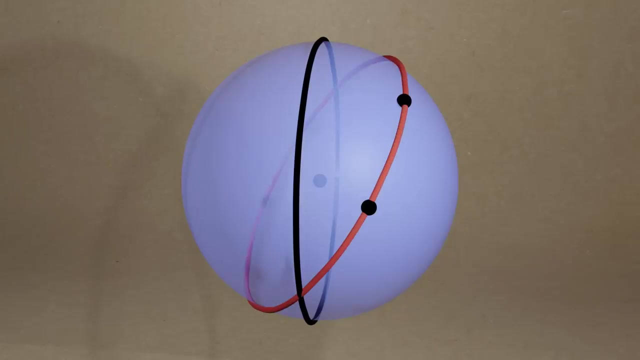 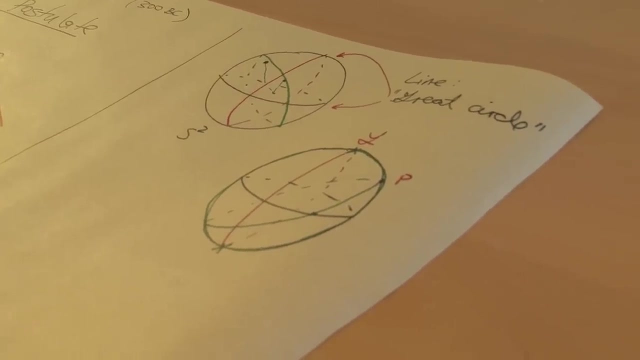 OK, so maybe, maybe we draw the line segment or the whole line that goes through P and then another point over here. OK, we draw it. Not good, No good. So it turns out that what happens in the Two sphere is that there are no parallel lines. 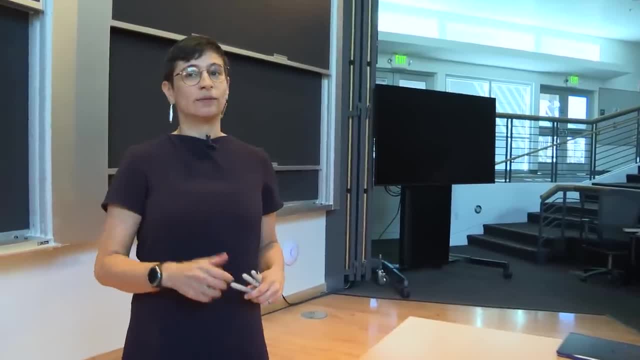 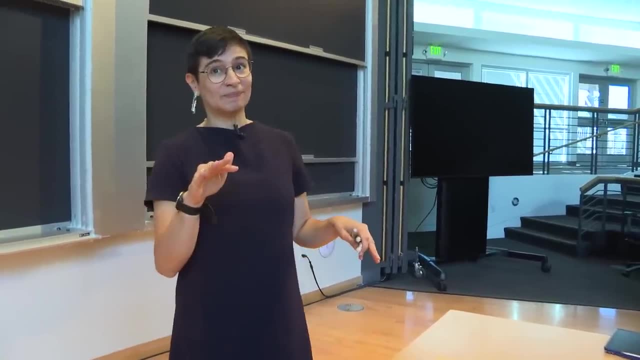 So before we say that in the plane there existed one and it was unique. So here we don't even have that first part of existence, We're done OK. but I mean, that's not, that's not Euclid's fault. 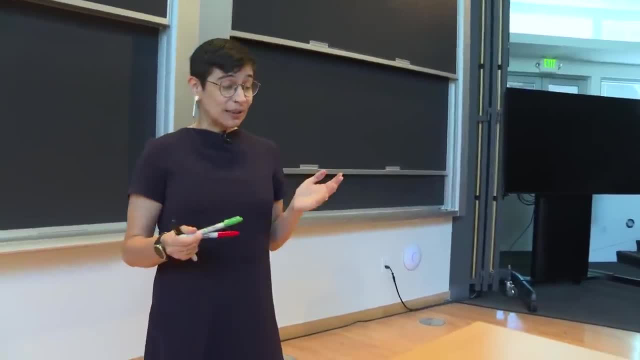 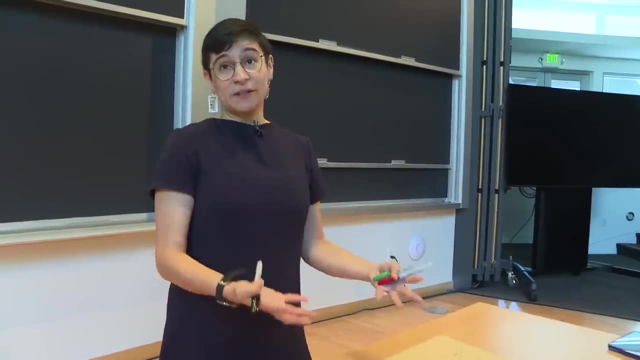 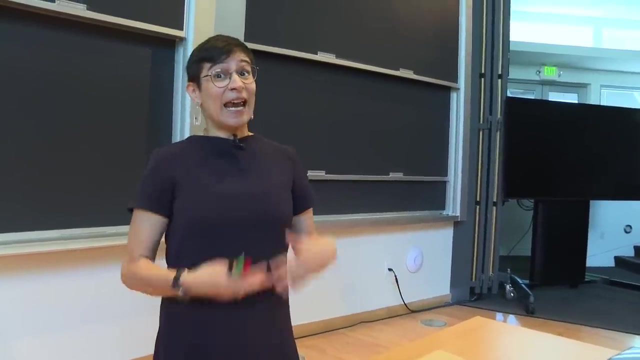 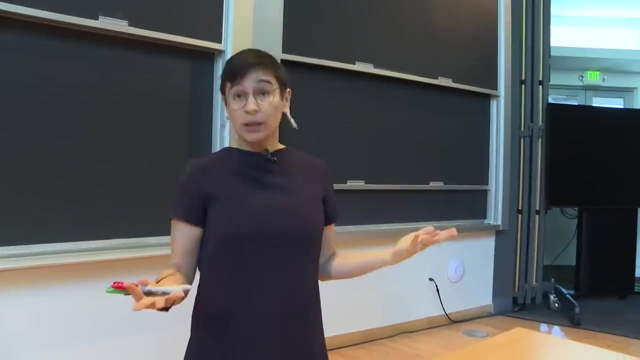 He wasn't talking about. No, no, no, no, no, no, absolutely not. It's actually kind of interesting because there was a lot of research being done in the geometry of the sphere, or trigonometry maybe to be more precise, because people needed this for navigation and for astronomy or astrology. for some people to you know, like everything that had to do with the skies was a sphere. 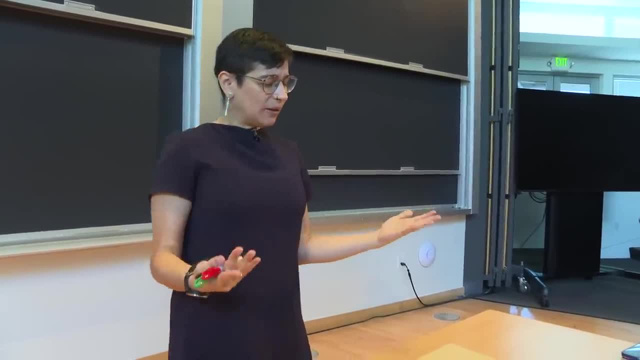 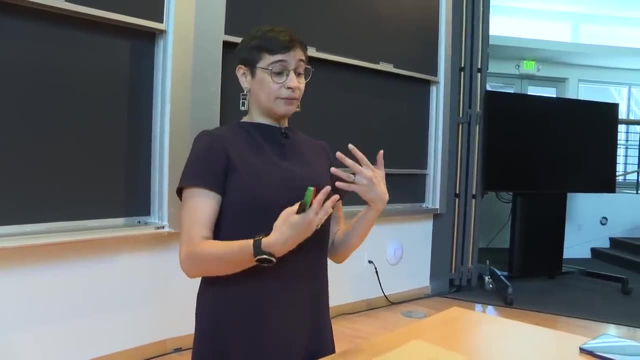 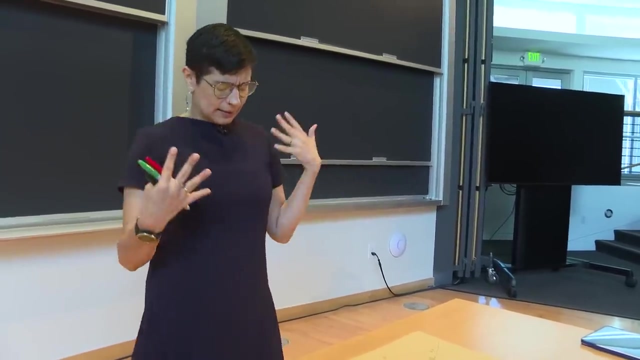 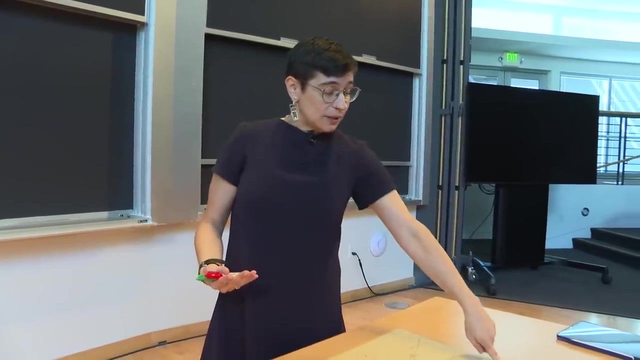 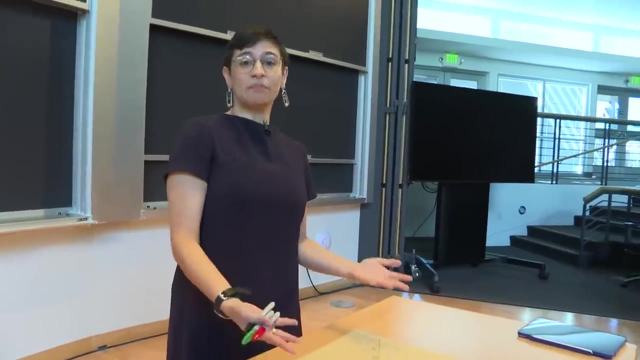 So there was a lot of knowledge, but somehow nobody thought that we could think about these two spaces as similar as both sharing a set of rules. Right, It wasn't until maybe later that we, And In the 19th century, that there was an upheaval in geometry, when we realized that in fact, if you consider the first four postulates of Euclid, there are other models where you can do geometry that holds, you know, that has those four rules, except for that fifth one. 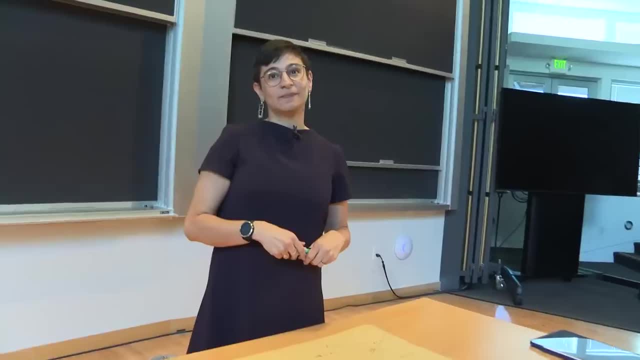 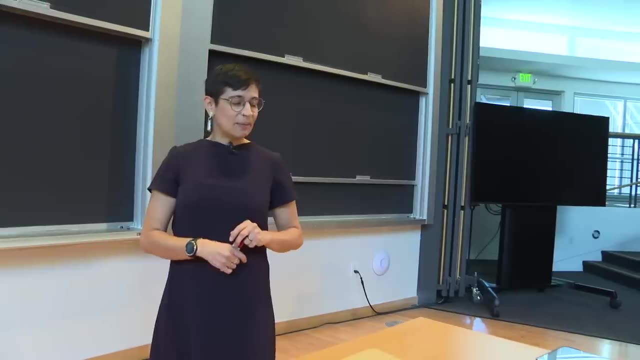 So that? so his first four rules hold up in other spaces. Yeah, This is the one that doesn't transfer across. Yeah, You know, maybe, To be precise, it might be a modern restatement of his axioms or postulates. 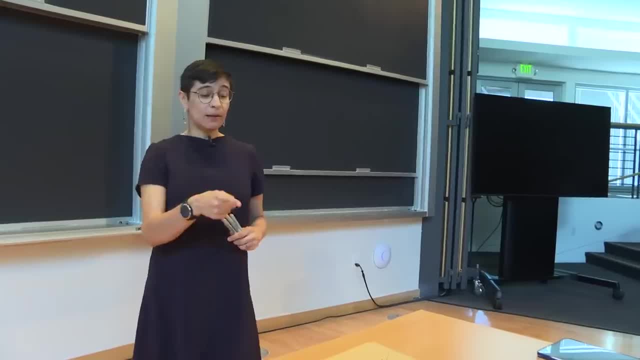 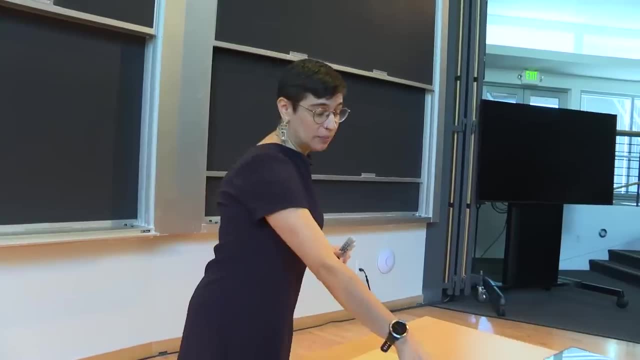 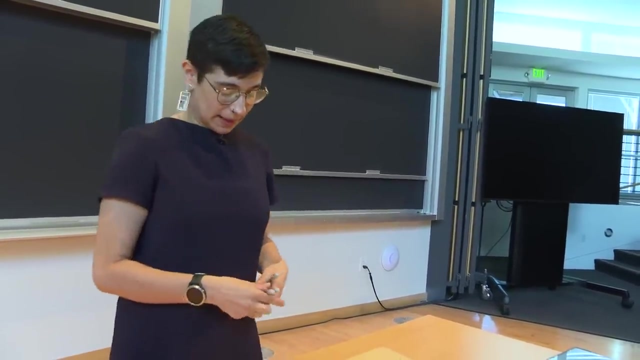 Right, Like we had to get rigorous. The one model or the one geometry that people started to think about, to show that the parallel postulate was just not true in general, was not spherical geometry but hyperbolic geometry. This is going to be a disk. 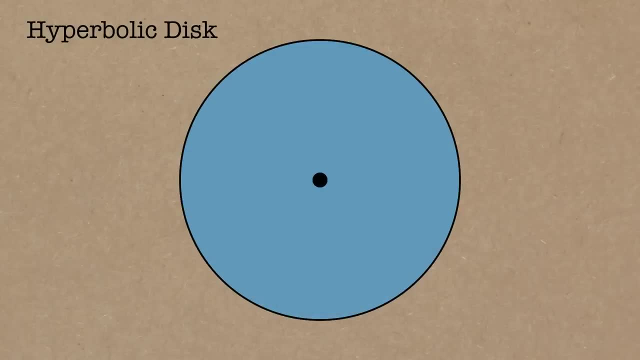 Let me draw the center, And again I have to tell you what it means to have a line. So a line, it's either going to be a straight line that goes through the center or, if I move a little bit away from the center, it's going to be the segment of a circle that is orthogonal to the boundary circle of the disk. 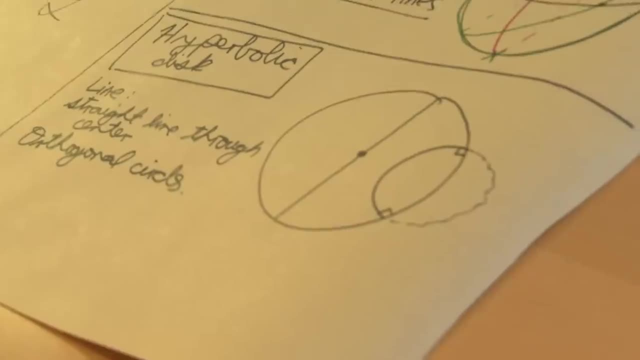 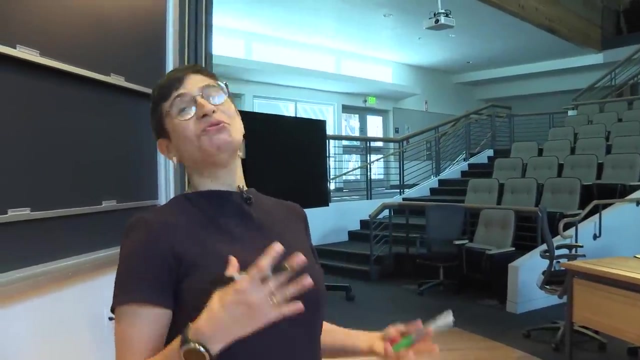 So are there parallel lines, Right? Well, in this case we are going to Have parallel lines, but we're going to have too many, So that's sort of like the other problem, right? Like we said, there exists and is unique. 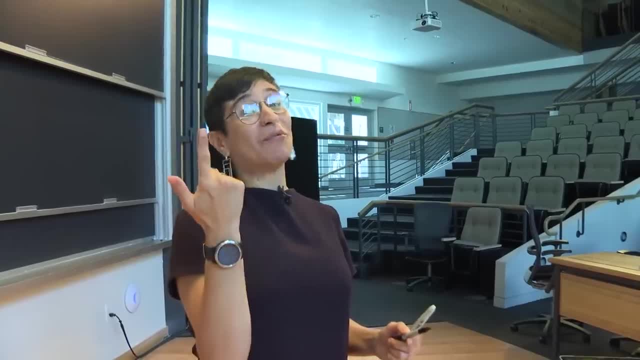 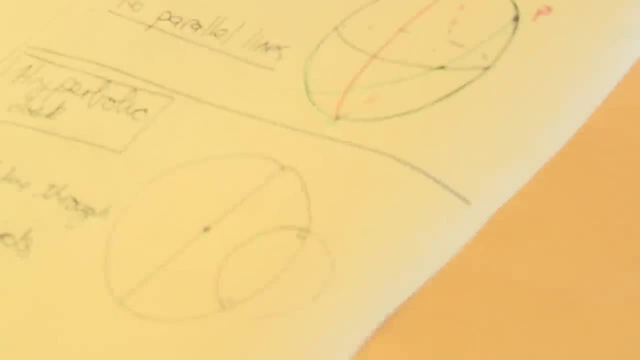 We already saw a place where they do not exist. Now we have one where they do exist, but they're not unique. So what happens here is um. so let me say again that this is my line L- why not? And let's say this is my point P. 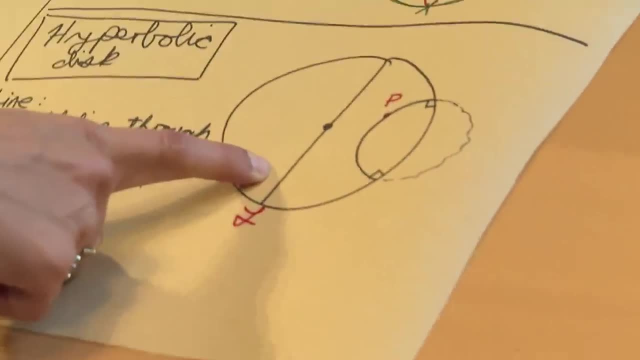 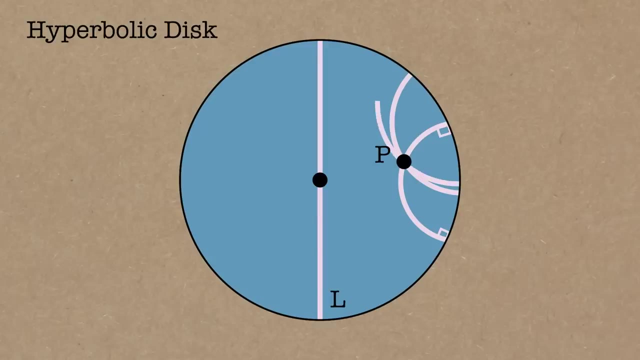 Well, that's one line that goes through. P Doesn't intersect, L- great. but I can draw more. I can sort of move my circles. I could just do many, many more, because in fact there are going to be infinitely many. 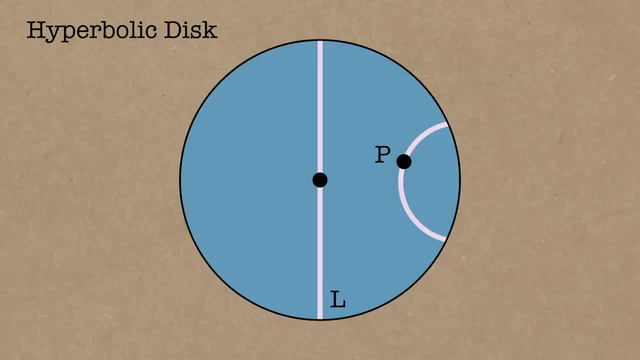 So the length, here again you know, going back to this distinction between a line, segment and a line, this circle is a line. It sort of looks like it's like finite right, Like here a line is, like the one that extends forever. 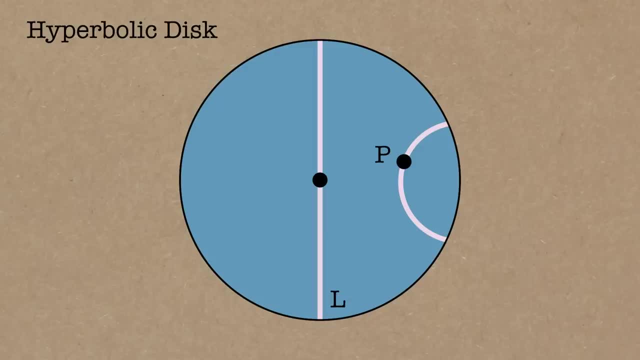 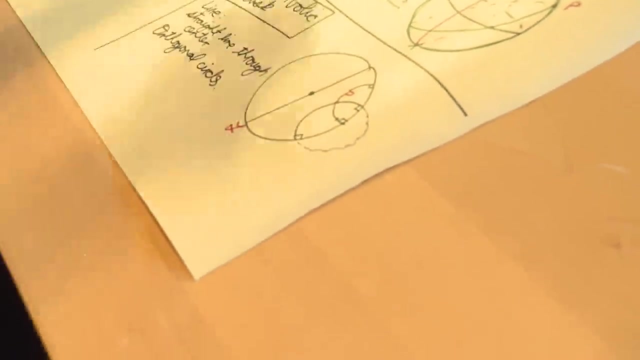 The way we measure distances here Is such that if you have two points that are very close to the border, these two points are very, very, very far away from each other, even though you know, like we're looking at it and if we were using the distance measurements that we had in the plane, they look very close to one another. 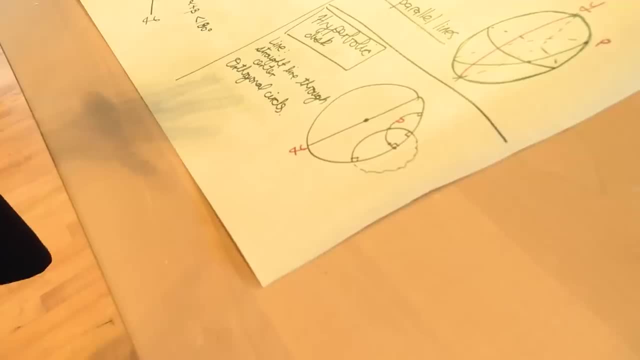 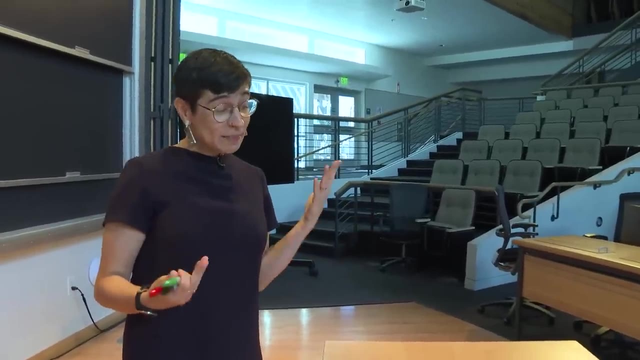 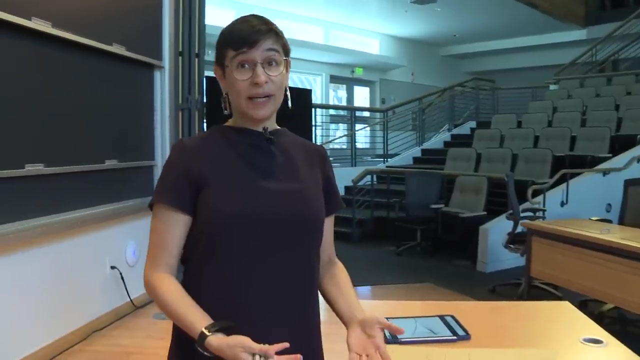 But the way we measure things in this new geometry makes them be very far away. This postulate has failed us again. Yes, exactly, Except here. And you know, it failed us in the sense that it it doesn't hold right. 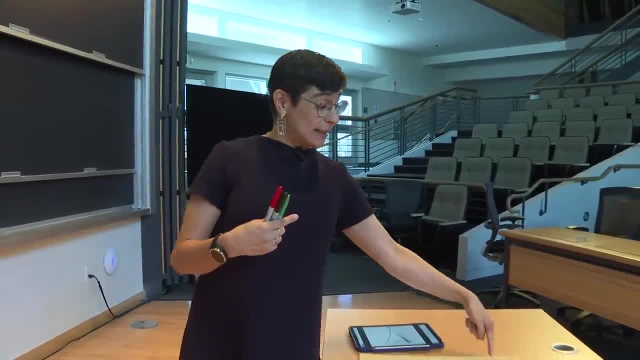 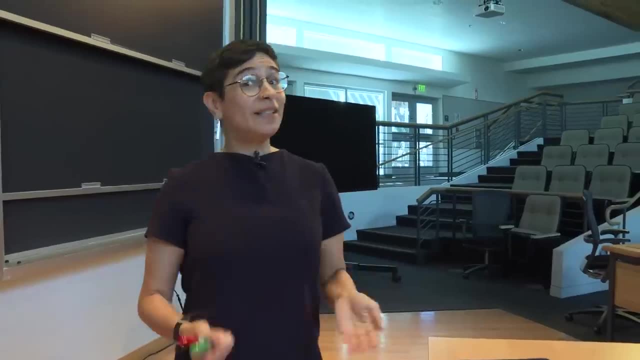 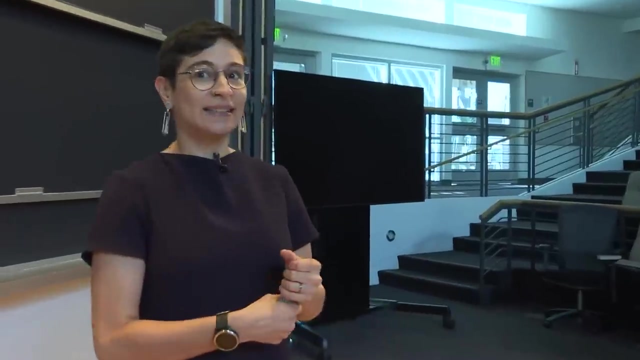 So that immediately means that it it is not a consequence of the first four rules, which was actually a question that people had for a very long time. Could it be derived from the first four postulates? And now we see that's just not the case. 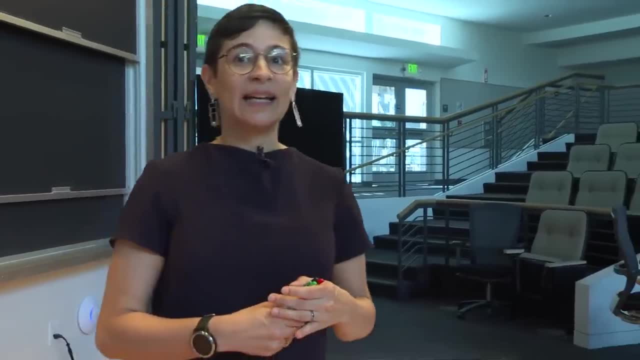 And clearly this fifth one was a bit of an add on. It's not part of the family. It's not part of the family. No, no, not exactly. And in fact, can the can the other four be derived from each other?